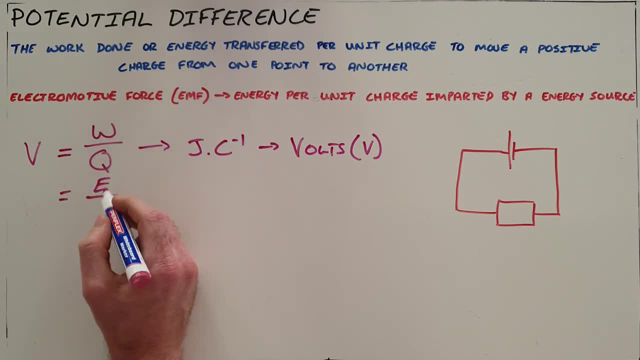 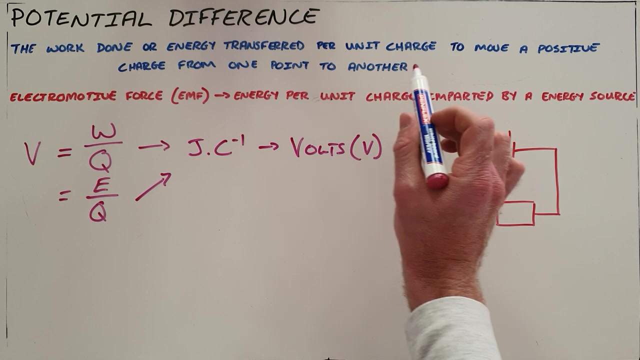 are interchangeable in this case, so the formula can either be w over q or also e over q, but both of them still give rise to joules per coulomb, which is then measured in volts. the second part of this definition, which is also important, is per unit charge: to move a charge from one point. 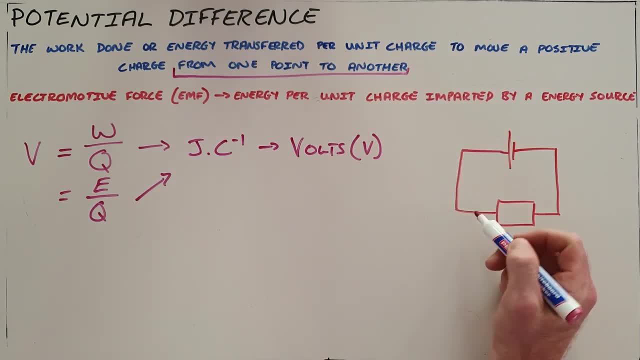 to another. now this specifies that it's the work done per coulomb of charge between two points. so it is essentially measuring the amount of energy that the current value of a products motor освathy increases. essentially because what that tells us is: firstly, it tells us why it is necessary for 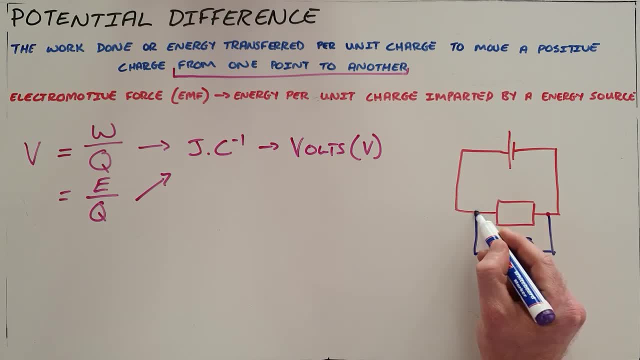 a voltmeter, always to be connected in parallel over a circuit. because what that voltmeter is doing is, it is measuring the amount of energy that is used between one point in the circuit and another point in the circuit that each coulomb of charge is using to get through that. because we know that. 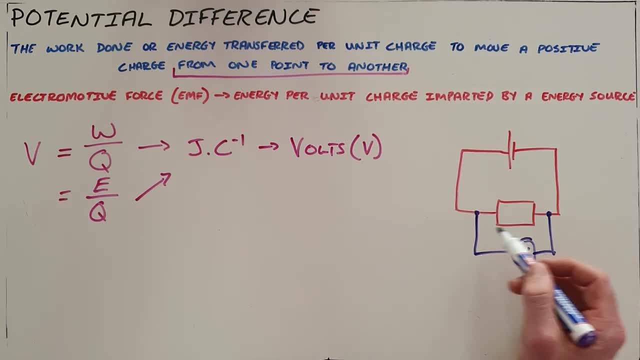 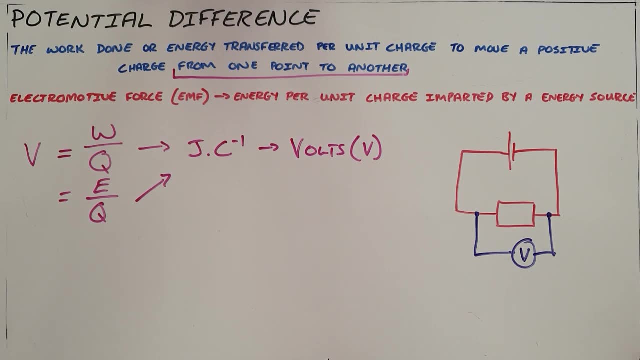 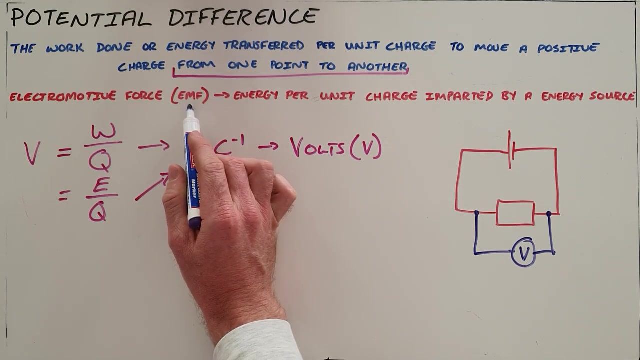 resistors slow down current in the circuit, thereby using up energy to pass through that resistor. It is also important to notice the difference between potential difference and electromotive force, or EMF, which is the energy per unit charge imparted by an energy source, and that is an energy. 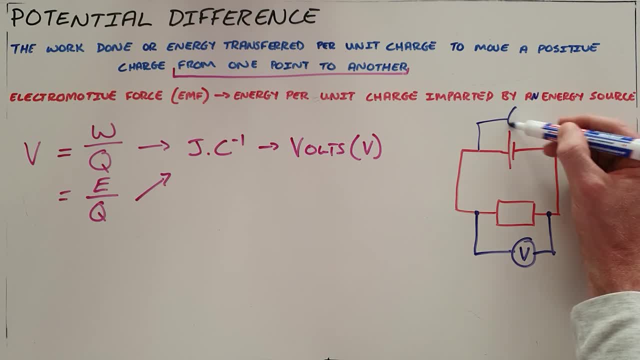 source only. So the EMF that is measured across a battery would also be its potential difference. but EMF refers specifically to energy provided by energy sources, where a potential difference refers to the amount of energy that is used per coulomb of charge to move a charge through any part. 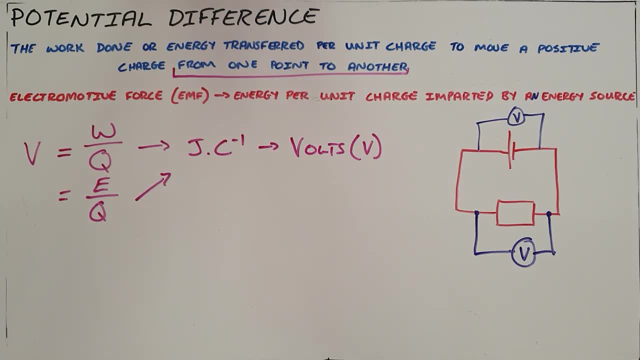 of a circuit. A typical question on potential difference would be something along the lines of the following: This resistor over here is found to use 12 joules of energy for every three coulombs of charge, so every three coulombs of charge that moves through. 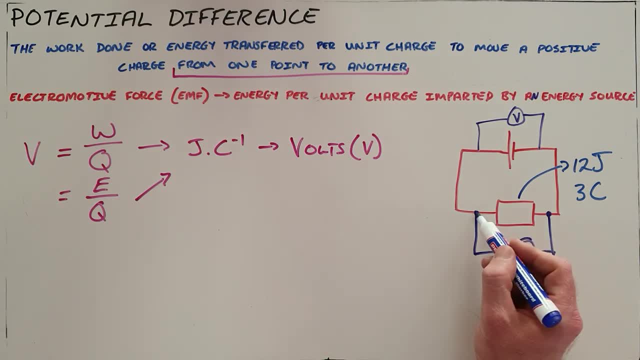 there uses up 12 joules of energy. What is the potential difference across that resistor? and we can say that V is equal to the amount of work that is done divided by the charge, and that is 12 joules divided by 3 coulombs of charge.